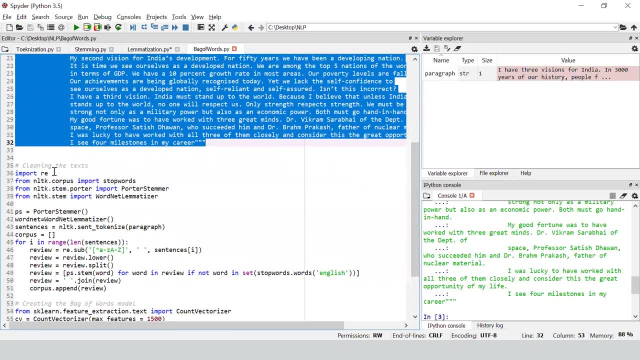 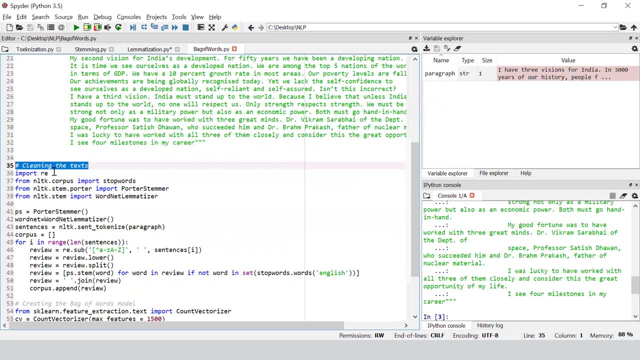 Okay, so for that I'm going to, first of all, I'll just call the first step as cleaning the text. okay, In cleaning, I'll be doing the lowering part also. First of all, I'm going to import the RE. 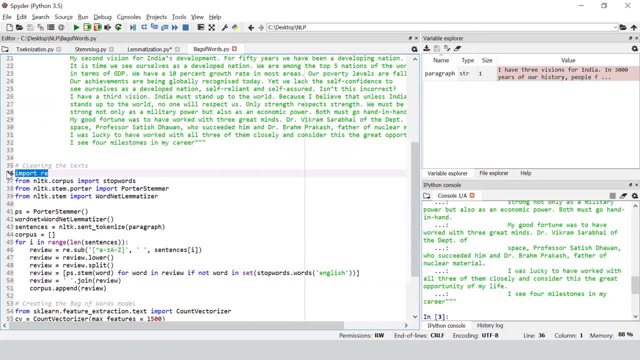 RE library is basically for regular expression. Guys, these all steps are very important because this helps in the cleaning of the text. Cleaning of the text is basically removing stop words, removing comma, full stop, lemmatizing it or stemming it, or you're trying to lower the sentences. 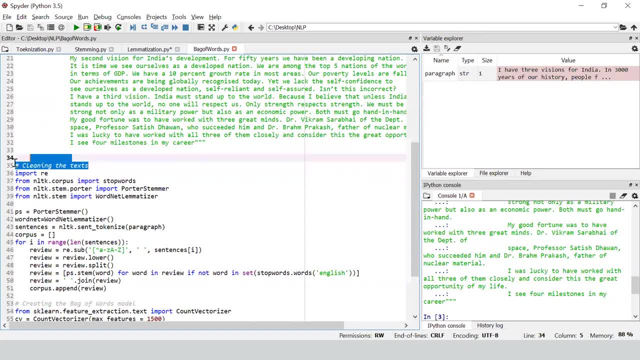 All those things. These will be actually included in this particular topic, that is, cleaning the text. So first I'm going to import the regular expression library- This is RE, okay, This RE library. Then I'm going to import the stop words. 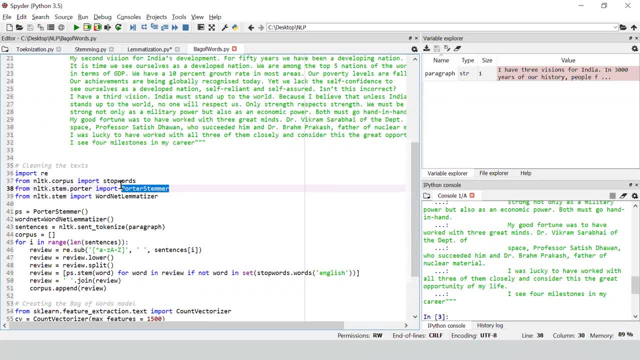 Then I'm going to import the porter stemmer. Porter stemmer is basically for stemming purpose. okay, Then, if you want to use stemming, you can import porter stemmer from nltkstemmerporter. Otherwise, if you're using lemmatization process, which we have discussed in the previous video, 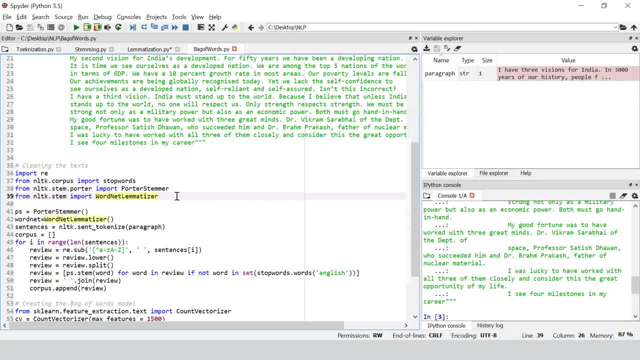 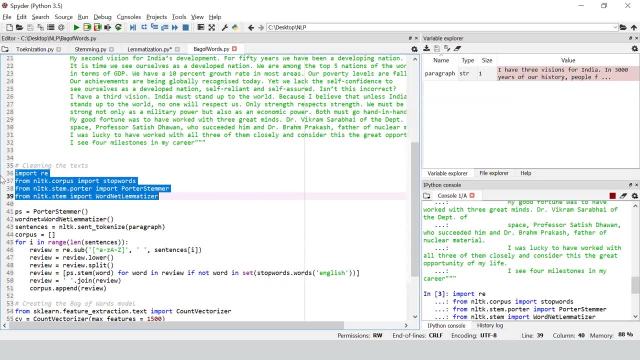 you can use nltkstemmer And you can import this particular library. So let me just execute this all statement and import all the libraries. So once I import all the libraries, then I can create the object for this libraries and play with it. 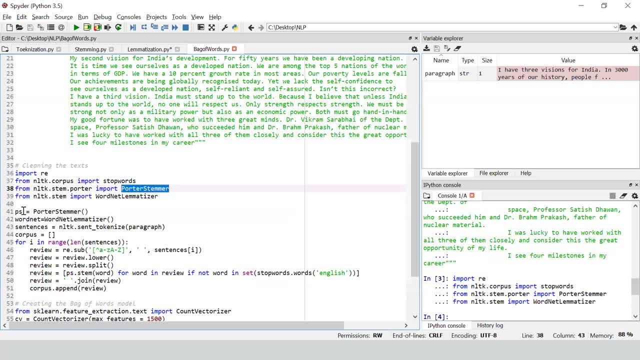 Now my next step is that, for the stemming purpose, I'm going to create my object, which is PS Okay, And this will be responsible for doing the stemming functionality. So let me just execute this First. I'll do the stemming. 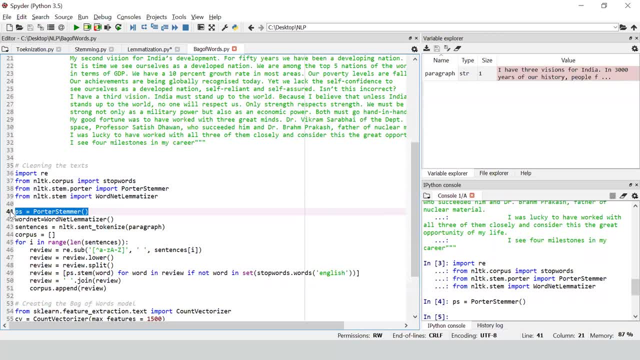 Then I will do the port lemmatization and I'll show you the difference. That's how it looks. Okay, Then let me import. sorry, let me create the object for lemmatizer also, which is from WordNet lemmatizer. 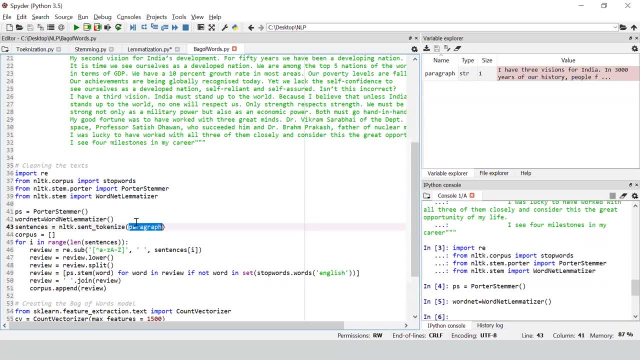 Now, to begin with, I'm going to convert this paragraph into sentences and I'm going to use the sent underscore tokenize function from this nltk. Okay, So once I execute this, you can see that how many sentences will be created and sentences will be in the list. 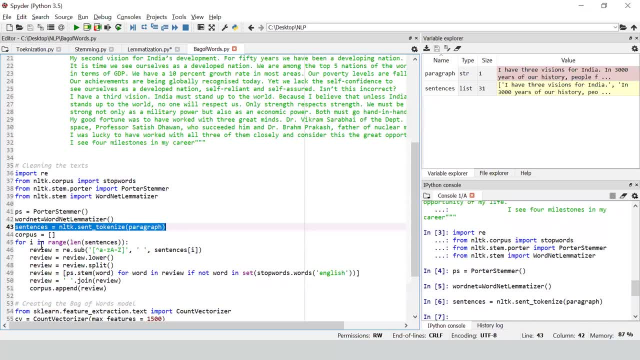 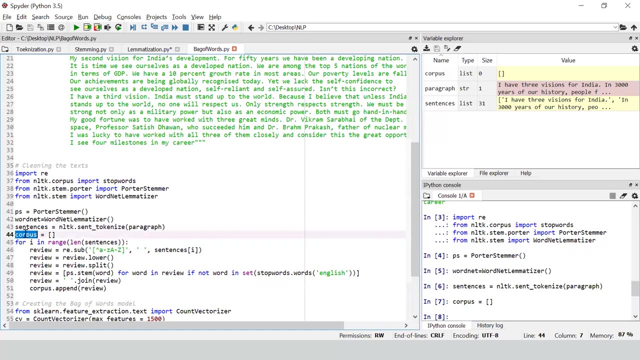 So I have 31 sentences in this. Okay, Now let me create another list, which is called as corpus. The reason why I have created this is because, after cleaning my text, I'll store all my sentences in this particular list, And then we can see the differences between sentences and corpus. 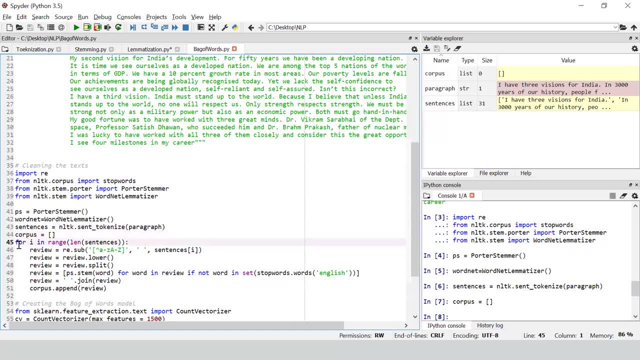 Okay, Now, this is the most important step with respect to cleaning. Okay, So what I'm doing is that I am iterating through each and every sentence So you can see, for I in range length of sentences. length of sentences is 31.. 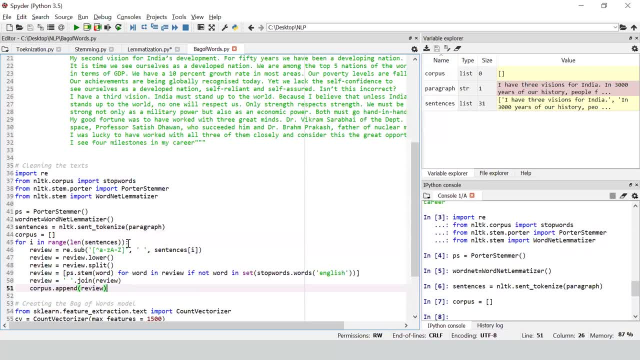 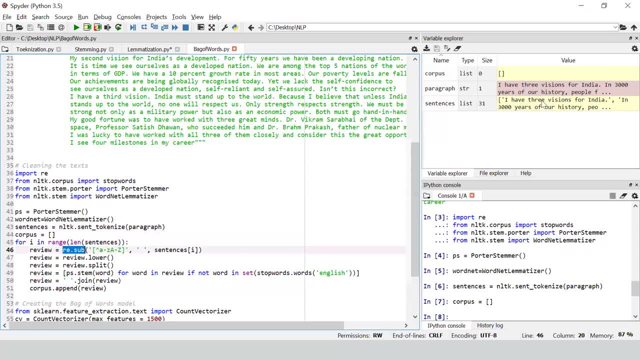 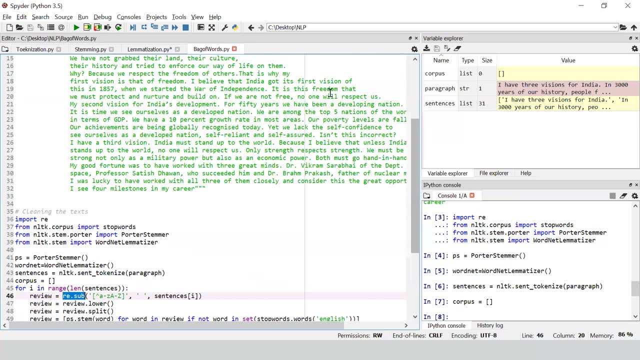 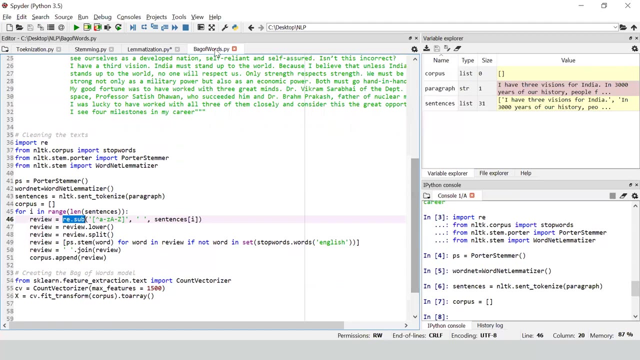 whole paragraph or all this. I'm cleaning up this whole sentences. I am removing all the comma, full stop, punctuation mark, question mark from this sentences that I have over here, because those are actually not responsible or not required for sentiment analysis. So what I'm going to do is that I am going to remove all those things. 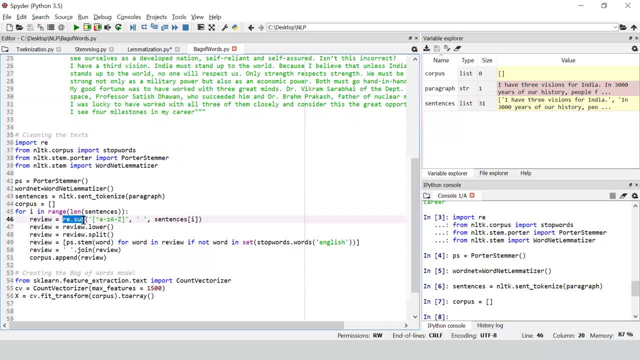 So for that I'm going to remove all those things. I'm using a regular expression: dot, sub, sub is a method where I'll be replacing all my other characters other than a to Z and capital- A to Z- That is my words- and characters- with spaces. 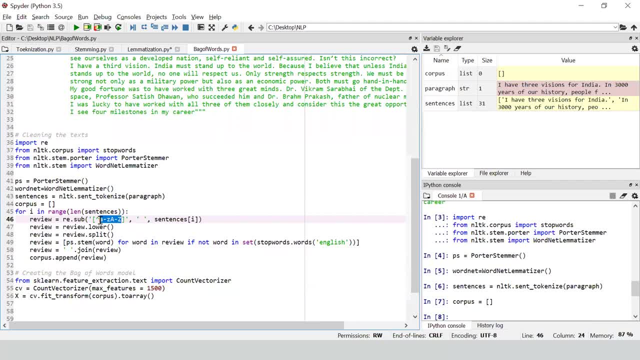 Okay, Apart from all these words, I'm replacing everything. Okay, This, this symbol, is not symbol. Okay, Apart from this, this particular words that I have, that is a to Z and capital A to Z. I'm going to remove everything with spaces. 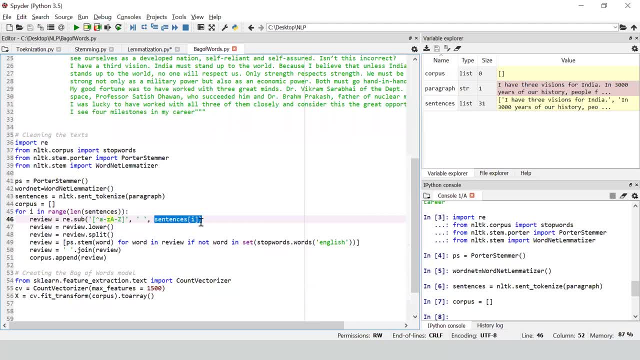 Okay, Okay, And- and I'm applying it to each and every sentences- Okay, Then, next step: I'm lowering each and every sentences, I'm lowering the words of each and every sentences, Then I'm going to do the split, split. 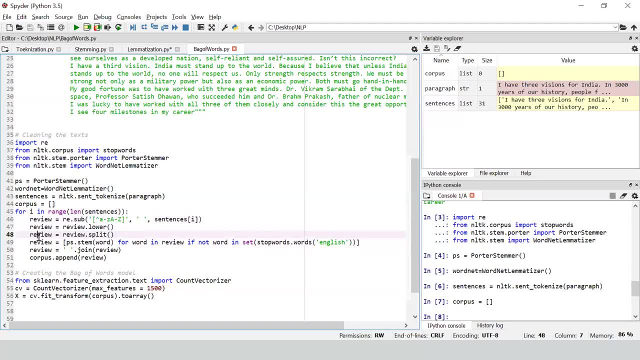 Actually, when I do the split of the sentence, I will be getting a list of words. So this review now will be having a list of words, And then my next step is basically writing the list comprehension that we have discussed in our previous example, which starts with: 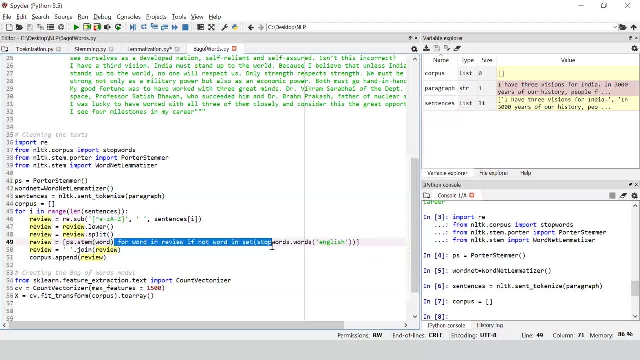 for word in review, if not word in, if the word is not present in the stop words, I am going to do something called a stemming. Okay, Here I'm using PS. PS object is for Porter stemmer, So I'm using PS dot stem. 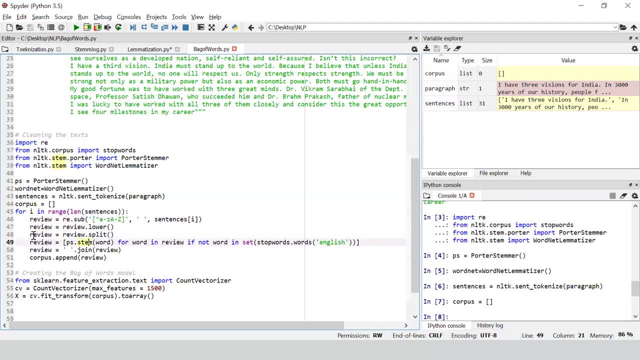 Okay, And this will be responsible for doing the stemming. And finally, I'm joining all this list of words of reviews into review and I'm appending to the list that I had created, which is called as corpus. So this is the whole steps. 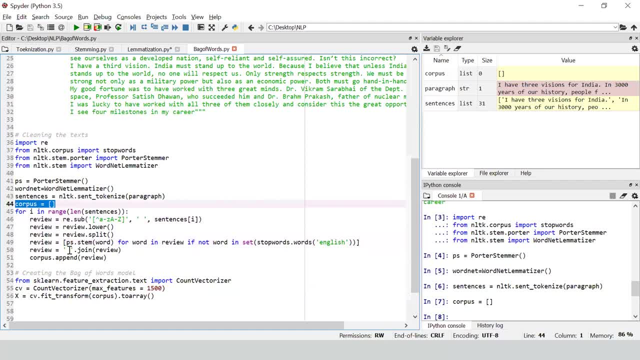 Again, guys, just go line by line, You will be able to understand it very perfectly. Okay, And this is the most important step, that is, the list comprehension. So let me just execute this whole statement along with follow: So everybody, focus on this. 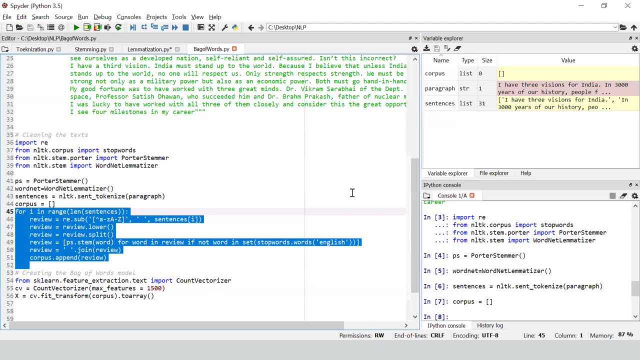 I have sentences here and then we can compare the sentences with corpus. Okay, So here it is. It will take some time to execute. Let's see how much time it may take. Here it is, It has got executed. Here is my corpus. 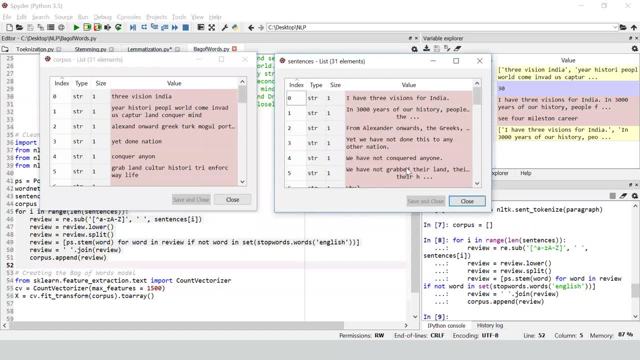 And here is my sentences. So this was my original sentences. after applying, after cleaning the text, after removing the punctuation, after removing the stop keywords and doing stemming right, I have all these words. that is great. Now see, in the first sentences I have, I have three visions for India, and over here it has. 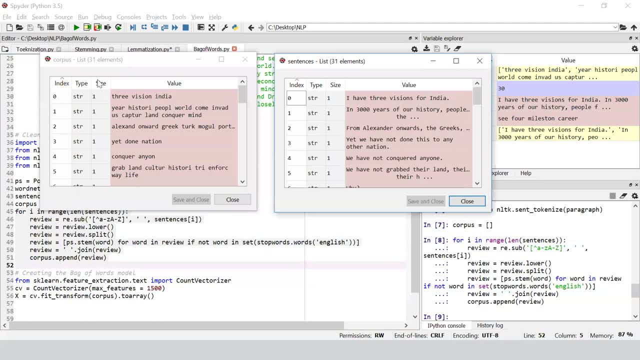 got converted to three vision India- Okay, You can see visions- has got converted to vision with the help of stemming. Okay, Then let us see another statement in 3000.. The years of our history that let us see the starting E, the eight and 3000 has got. 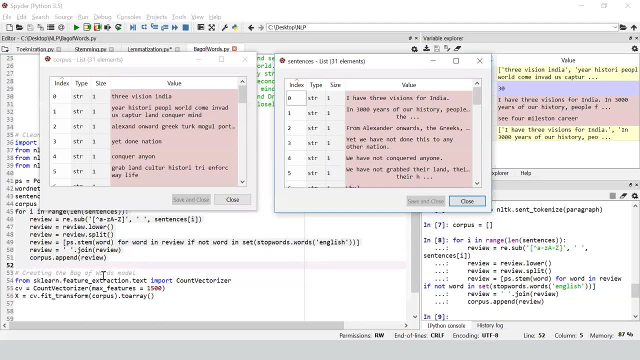 been removed, because we have just removed everything apart from A to Z. Okay, All the characters, but this years has got converted to year due to stepping at this history has got converted to something like H I S T O R, I. Okay, Now why has got converted to I? this will not form an appropriate meaning of a word. 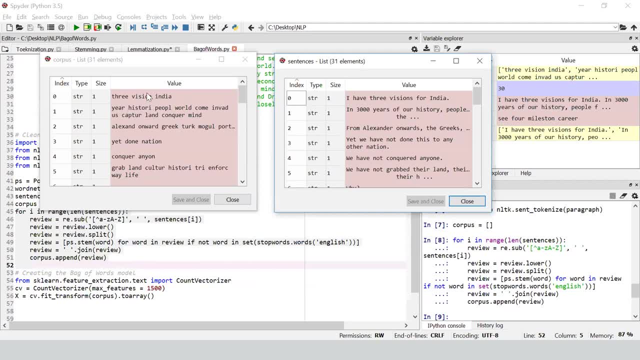 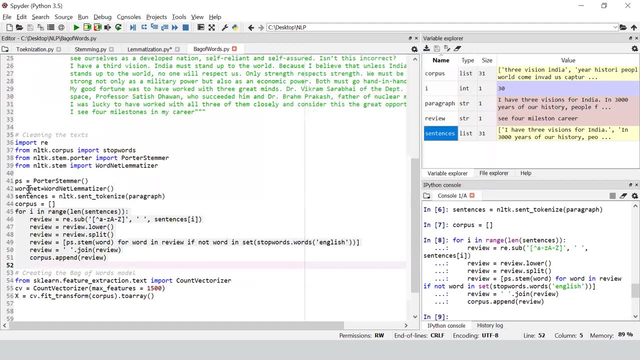 So the intermediate representation Of the stepping is not good, right, It may not have a meaningful word. So because of that, what I can do is that, instead of doing stemming, I will try to do something called as lemmatizer. 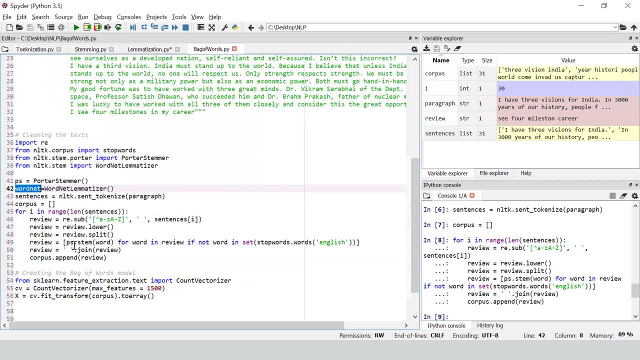 So I'll use this word net object, which I have created for lemmatizer, and I will write dot lemmatize. So I'll just replace P S dot step with word net dot lemmatize, and let me just do the same. 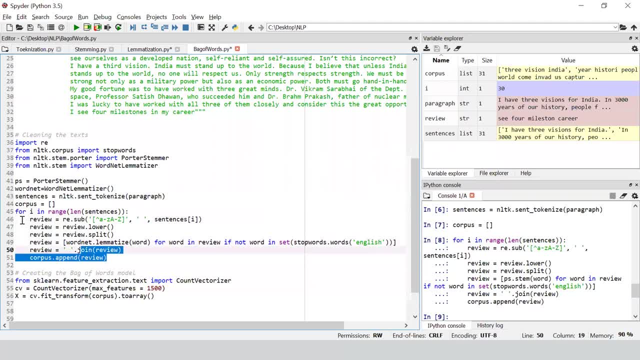 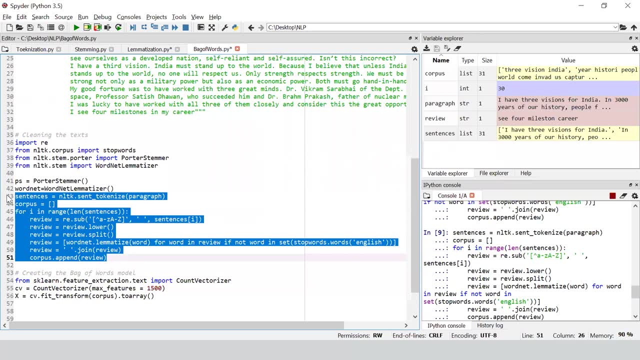 thing again. Okay, I'll just execute from the sentence And let's see how the difference, how we'll be seeing in this particular corpus. Again, it'll take some time. Uh, let us wait. Now it is done. So let us compare sentences. 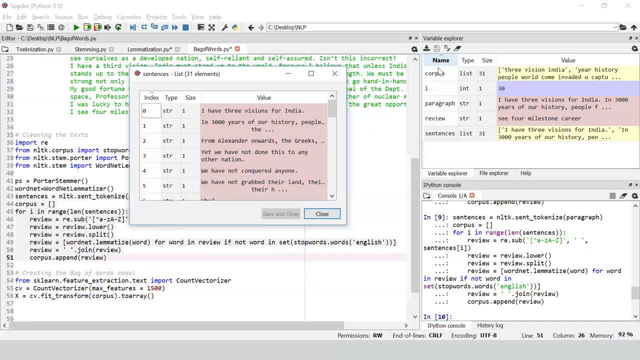 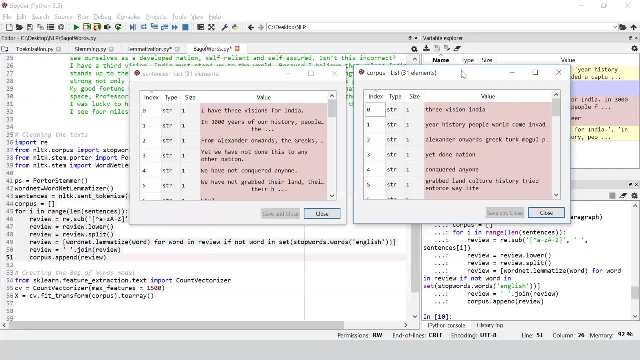 Okay. So this is my sentences with my newly corpus, where I actually applied, you know, lemmatization. before lemmatization, I've done the cleaning by applying stop keywords and removing the unnecessary words. Now you see this sentence, Okay. 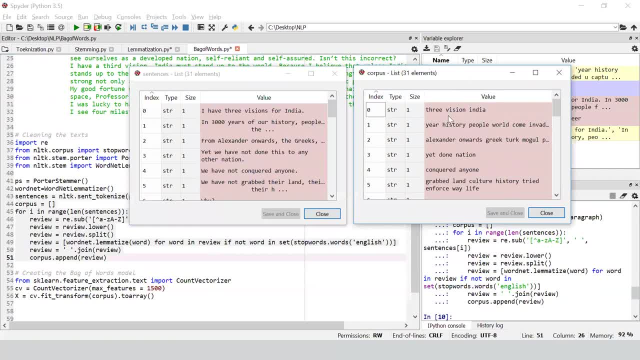 So I have three visions for India. three vision: India. This has got converted nicely. but in 3000 years of our history- you can see now years a year- it has got converted in lemmatization. history is history only. 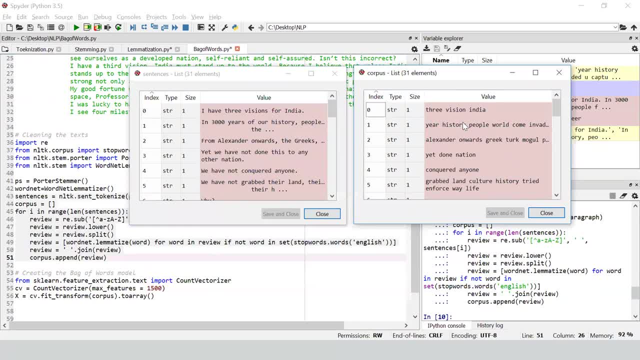 Okay, So lemmatization make sure that the intermediate representation will definitely have a meaning. Okay, So, because of that, lemmatization performs very well when compared to stemming, but usually lemmatization takes more time, And I've also shown you the differences between lemmatization and stemming in my previous video. 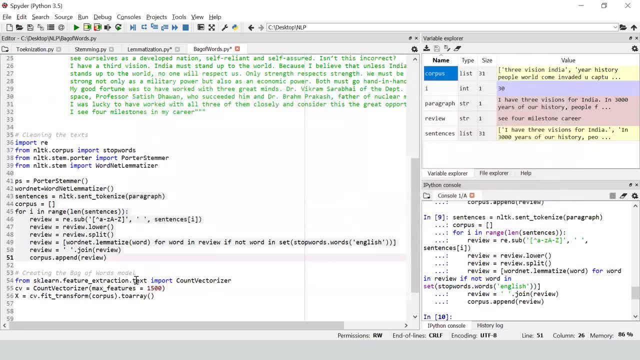 I will tell you about everything else. Okay, So I have two methods here and one method that is created. I've shown you a lot of different methods. You have the first method, document matrix. I am going to take you through it. 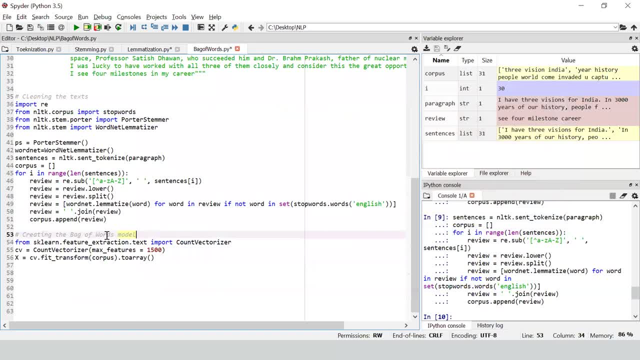 Let's start with the document matrix. Okay, So I am going to say that this is the document matrix, which is the bag of words. I am going to say the document matrix in this class. it has a document matrix and it has 4 words. 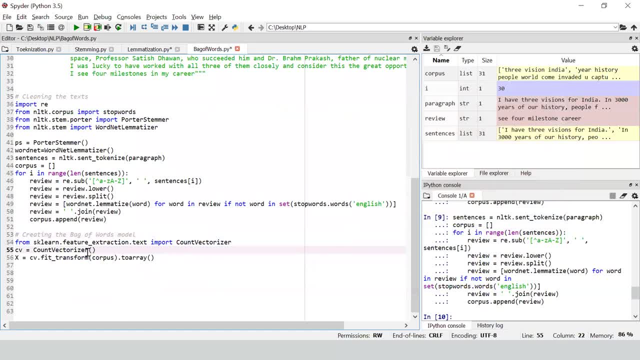 First of all, let me take a closer look at this document matrix together. So this is the document matrix. This is the document matrix that I have created in the class. Okay, Now the next step is creating the bag of words. right? 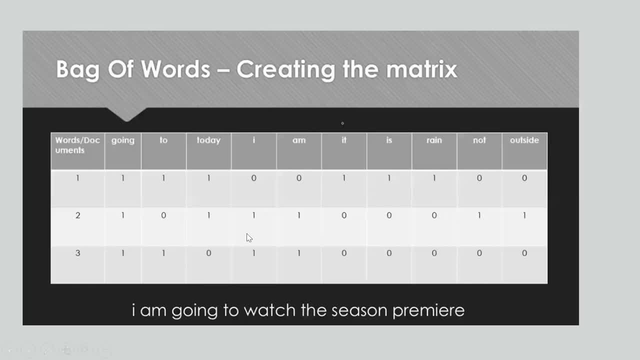 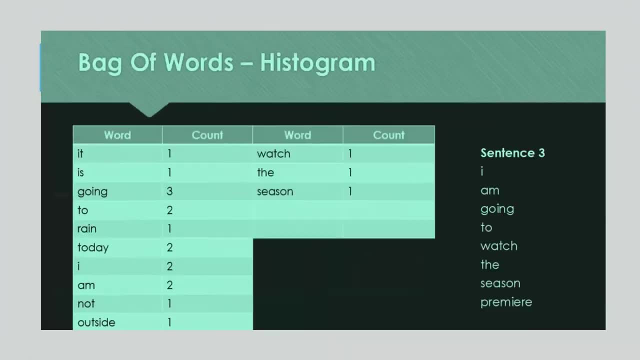 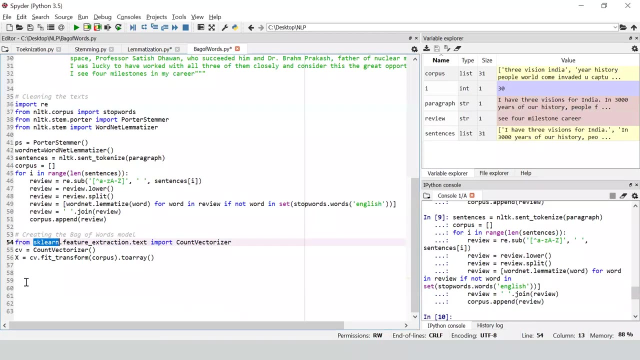 Now I told you, bag of words is nothing but the document metrics, document metrics all together. Okay, right, all these steps will be, I mean, from here. so basically, you know, if I take this histogram, histogram, taking histogram, then sorting the histogram, filtering the words, then creating the matrix, this all is done by this. 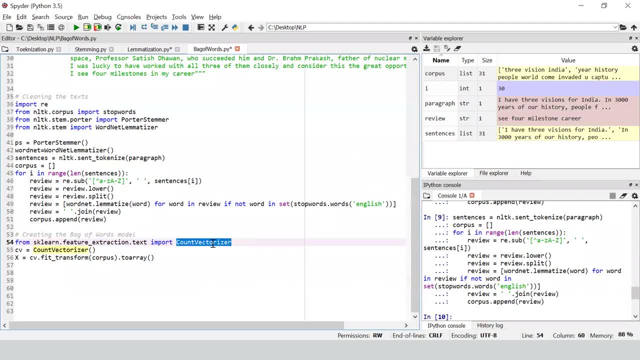 particular library which is called as count vectorizer and it is present inside sklearn dot feature extraction dot text. okay, sklearn is a very important- you know altogether- library because it has a lot of machine learning libraries. it has, you know, dimension reduction libraries, has data pre-processing libraries. so one of the data pre-processing library is something: 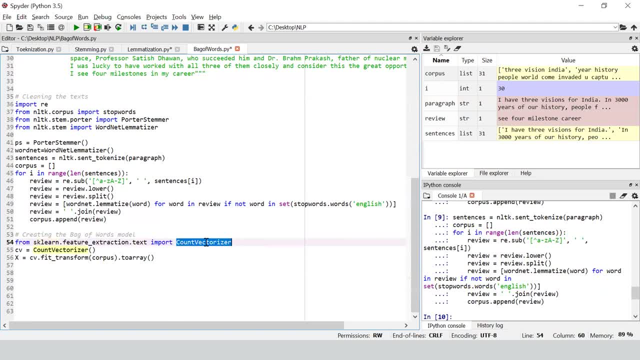 called a count vectorizer, which is responsible for creating the bag of word document matrix. so I'm going to import this particular library first. then I'm going to create the object for this little library, that is CV. okay, after I create the object, I just have to use something called a CV dot fit. 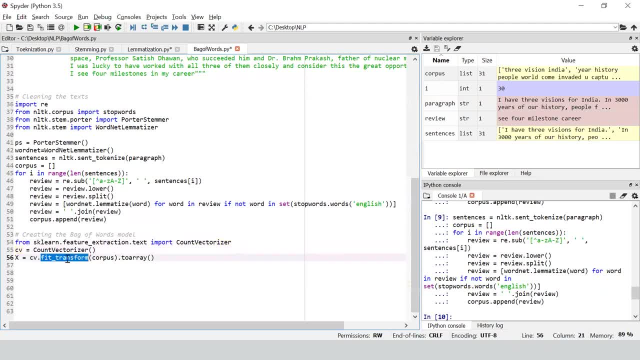 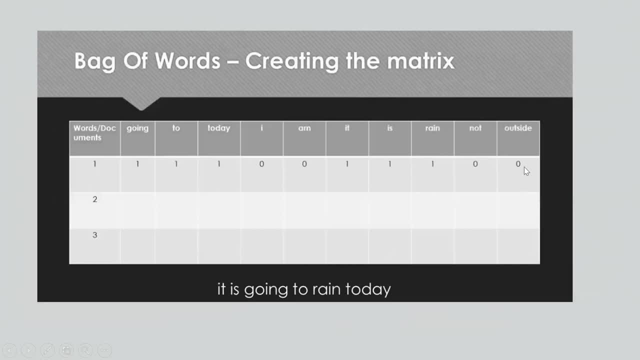 transform. fit transform will be actually responsible for creating the document matrix. so I'm going to import this particular library, which is called a count vectorizer, which is responsible for creating this kind of matrix, and finally we'll be able to get this kind of- you know- matrix getting converted into one zeroes. so we'll be using fit transform and I am 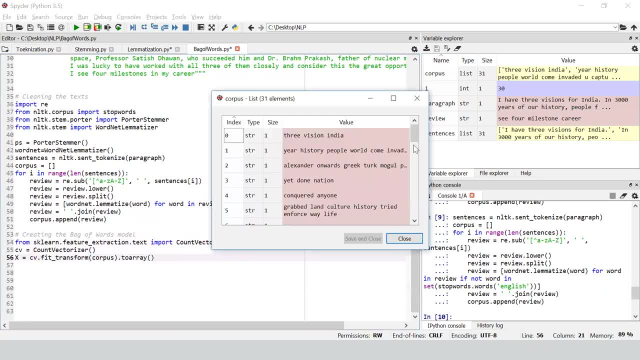 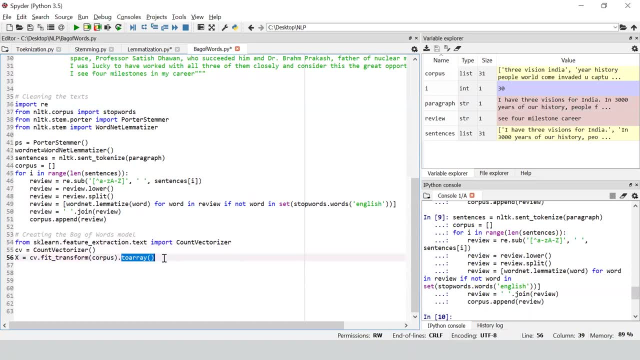 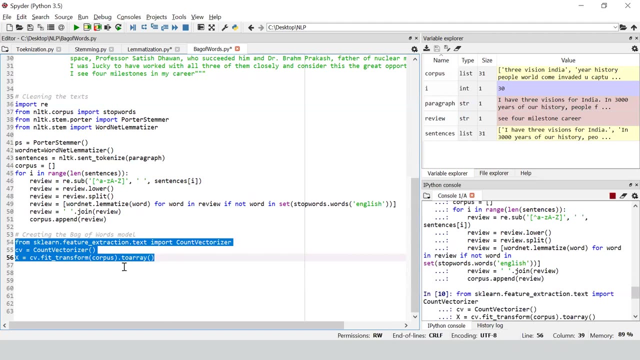 going to apply this fit transform on my new corpus that I have actually created. so here is my corpus and finally, I'm converting into an array so that I can be able to see it properly. so let me just execute this. now. you see this. I've named it as X. as soon as I execute all my text. 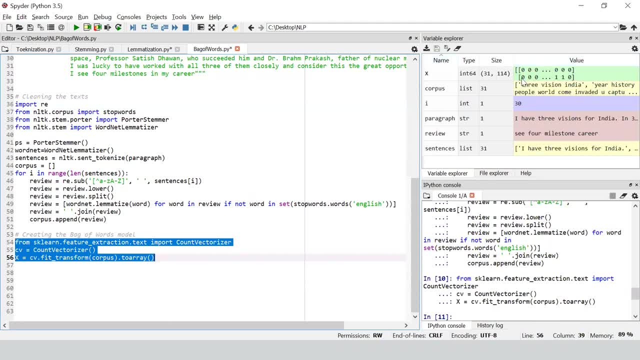 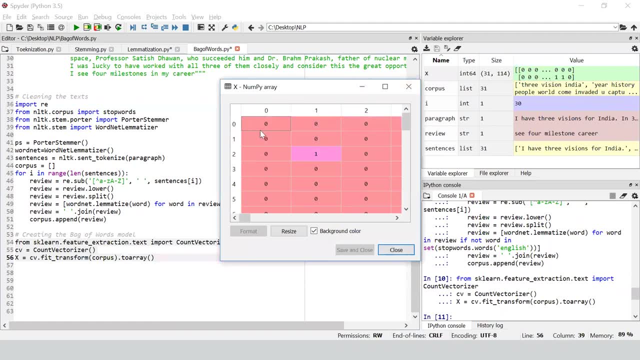 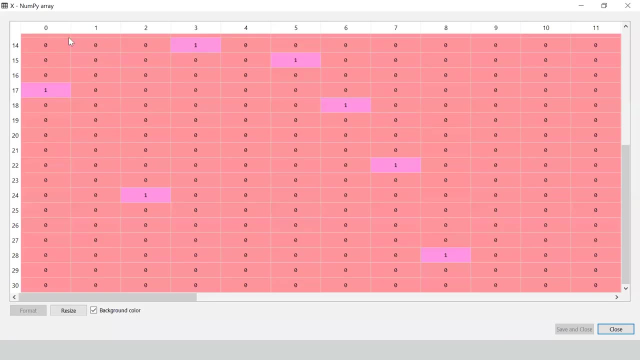 over here in corpus. okay, in corpus, now you can see that my x, you can see the dimension. it is 31 comma 114. 31 basically means that i have 31 sentences all together. okay, i'll just expand it and you, now you can see that for the first sentences, if the word is present somewhere. 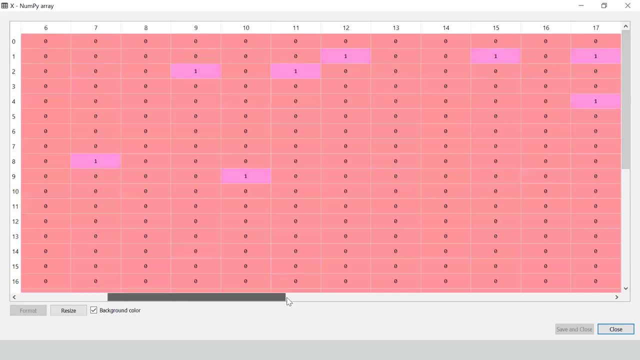 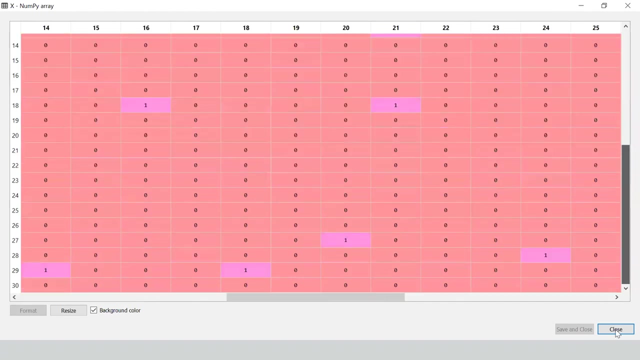 it will become one, otherwise it will be zero. okay, now you can see. just scroll down from left to right with respect to this. here you can also see two, because this particular word is present two times in this particular sentences. right, so all my 31 sentences over here has got converted into. 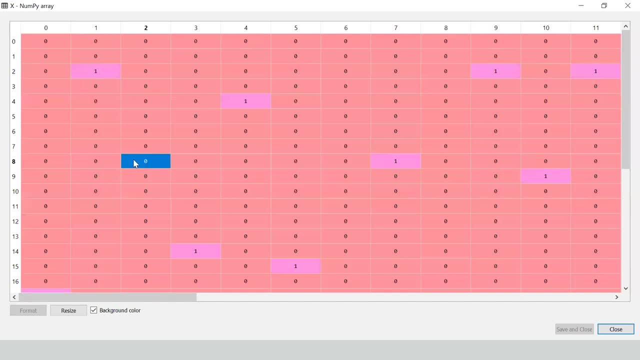 document matrix. now this is my input, guys. this i can provide it to the model. the model will be able to understand by seeing, wherever it is, zeros and ones. it will be treating that those words are actually present and it can apply some machine learning algorithm to find out whether we are. 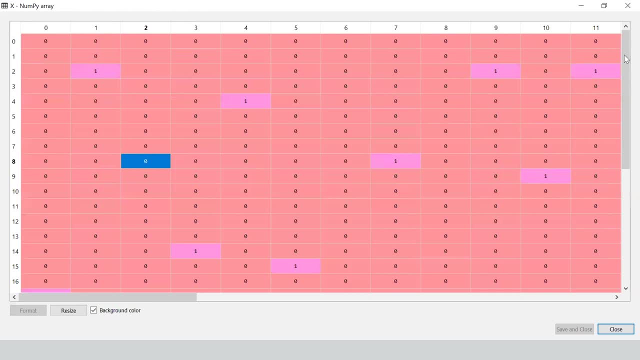 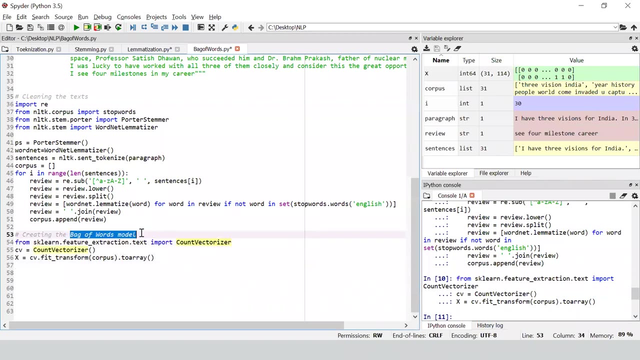 doing the sentiment analysis and where we can find a positive and a negative comment. so this is a perfect example of, you know, the count vectorizer, which is creating the bag of word models. so this was all about the class guides. remember the concepts. if you're not able to understand, just see the video from starting. 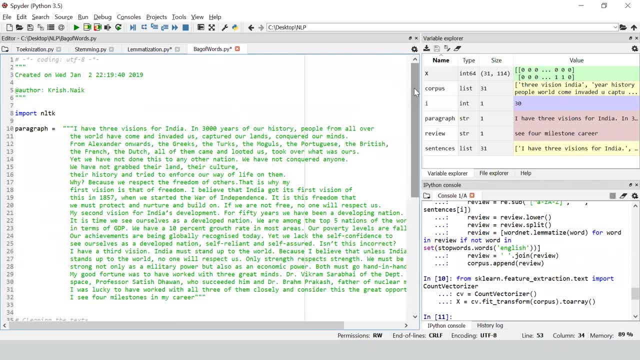 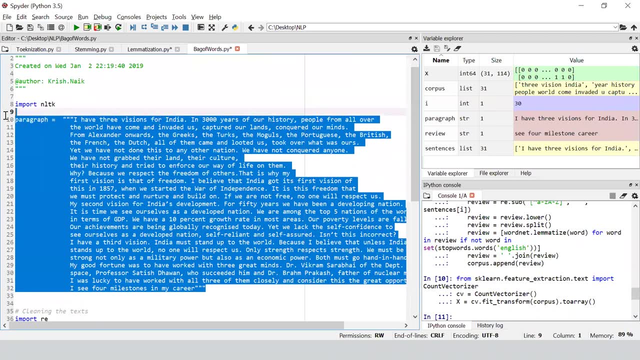 try to see step by step. so i try to see the text. i'll put this text in the github link. you can download it from there and try to you. you know, try to do the same example with different, different paragraphs that you have. just copy some paragraphs in wikipedia and 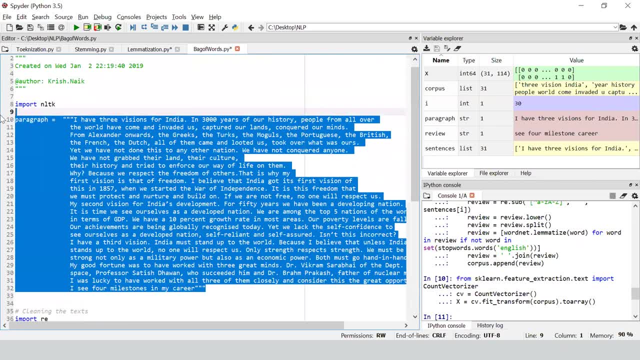 just copy some paragraphs in wikipedia. and just copy some paragraphs in wikipedia and just try to, you know, paste it and try to see it over there. okay, so i hope you like this video. if you have not subscribed to channels, please subscribe the channel. i'm continuously uploading. 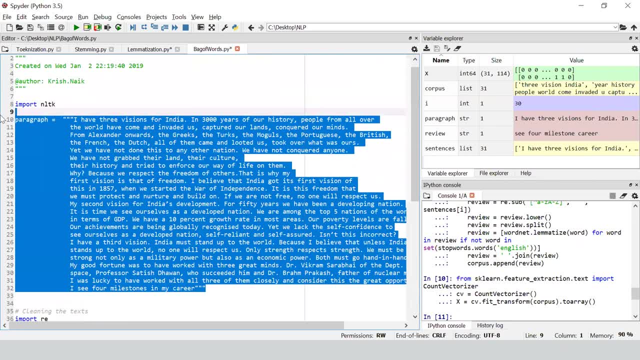 videos with respect to different different topics. i also have different different playlists- nlp- sorry, nlp- is one of the playlists. i also have a playlist on machine learning, on statistics, on feature engineering. so all these things, i'll be slowly, slowly, uploading those playlists and those playlists will be getting updated day by day. okay, i hope you like the video guys. 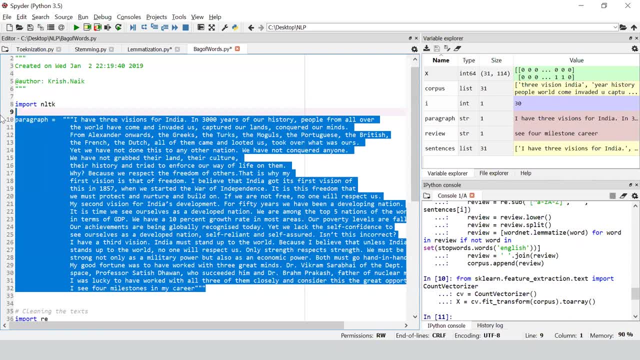 if you have liked the video, please share with your friends who are in need of data science because i'll tell you, after four to five years, everything will be like. many companies will be working extensively on data science. many companies are currently moving slowly, slowly, to data science. 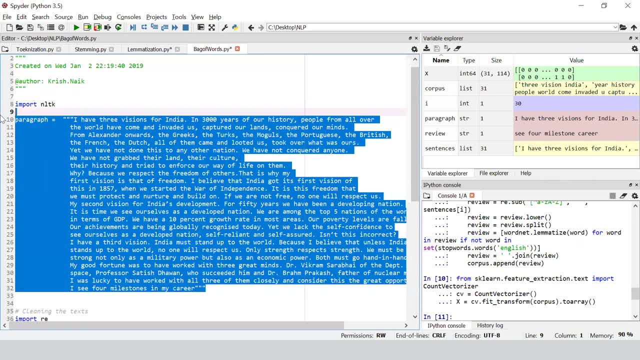 and they are requiring a huge workforce population. so please, uh, share with your friends who are in need of data science tutorials and uh, yes, i'll see you in the next video. next video, we'll be discussing about something called as term frequency and inverse document frequency, which is a better 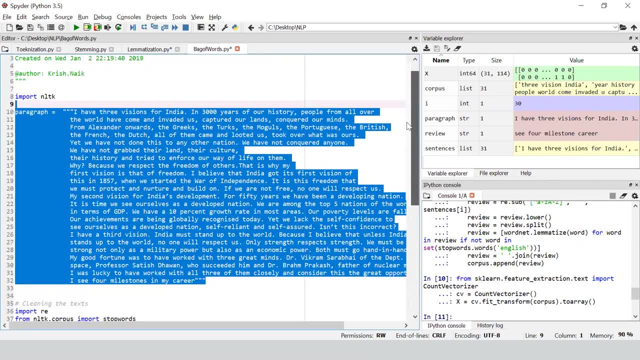 technique than bag of words, and i'll see you in the next video. next video, we'll be discussing about something called as term frequency and inverse document frequency, which is a better technique with respect to the bag of words. so i'll see you in the next video. till then, enjoy, have a great day.